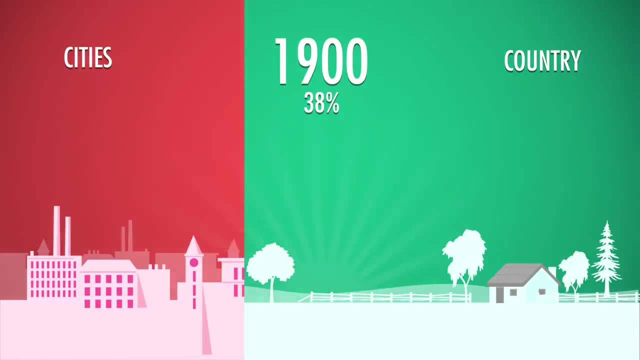 people. This rose to 18 cities in 1900,, with the percentage of urban dwellers rising to 38%, And by 1920, 68% of Americans lived in cities and 26 cities had a population over 100,000. 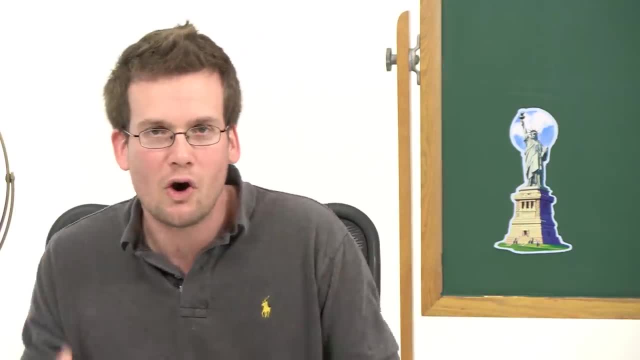 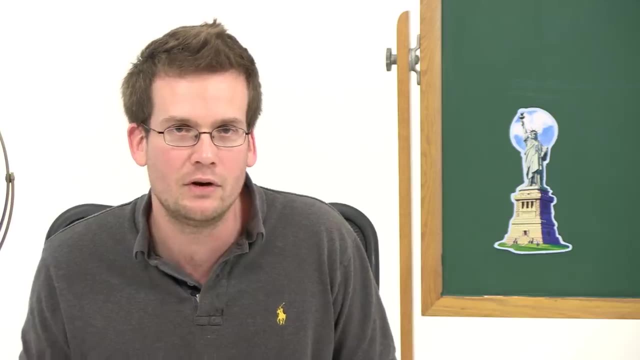 So in the 40 years around the turn of the 20th century, America became the world's largest industrial power and went from being predominantly rural to largely urban. This is, to use a technical historian term, a really big deal, Because it didn't just make cities possible, but also their products. It's no coincidence. 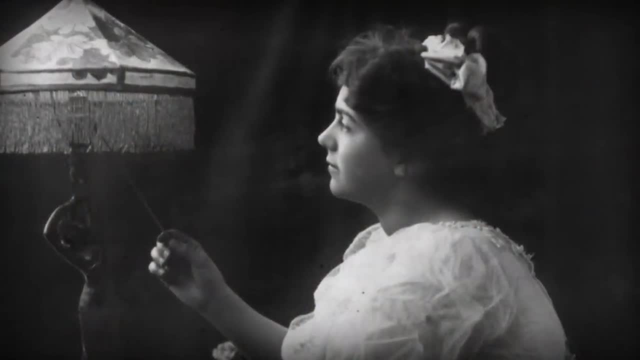 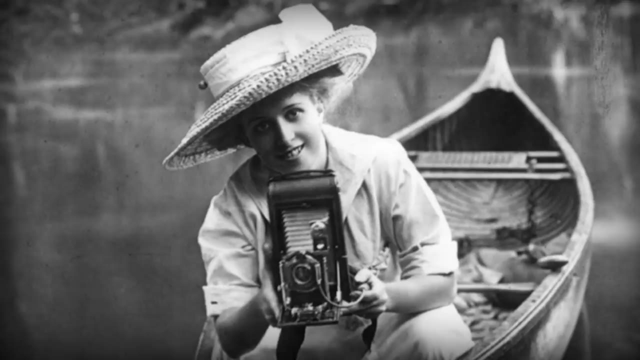 that while all this was happening, we were getting cool stuff like electric lights and moving picture cameras, neither of which were invented by Thomas Edison. I don't know if you've noticed, but suddenly there are a lot more photographs in Crash Course US History. 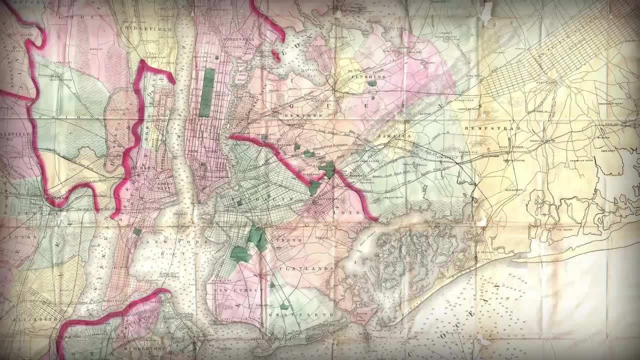 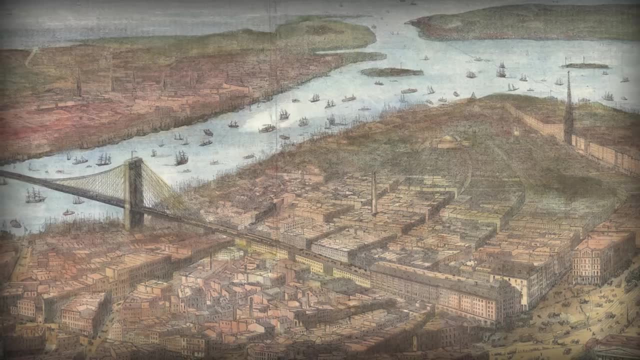 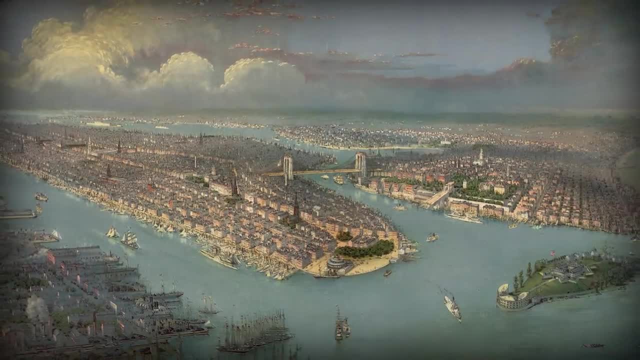 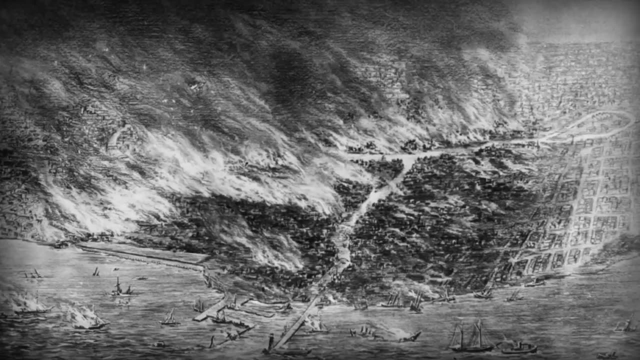 five boroughs had a population over 4 million. But while New York gets most of the attention in this time period and all time periods, since it wasn't alone in experiencing massive growth, Like my old hometown of Chicago, after basically burning to the ground in 1871, became the second largest city in America. 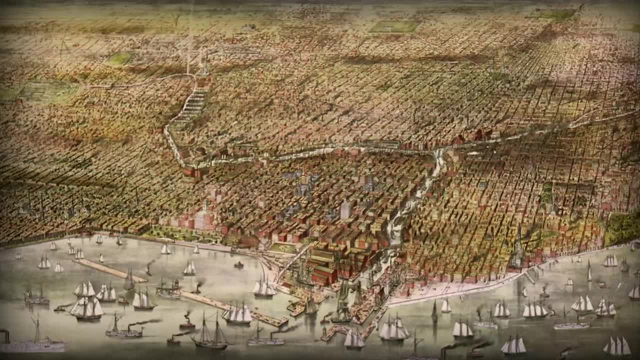 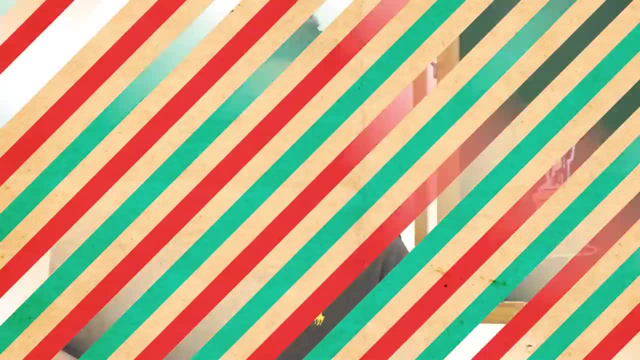 by the 1890s. Also, they reversed the flow of the freaking Chicago River, probably the second most impressive feat in Chicago at the time, the first being that the Cubs won two World Series, Even though I'm sorely tempted to chalk up the growth of these metropolises to a combination of better nutrition and better food. I don't think it's a good idea. I'm going to have to bow to stupid historical accuracy and tell you that much of the growth had to do with the phenomenon that this period is most known for: Immigration. 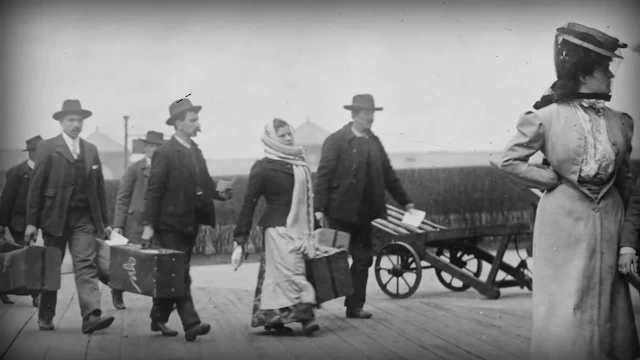 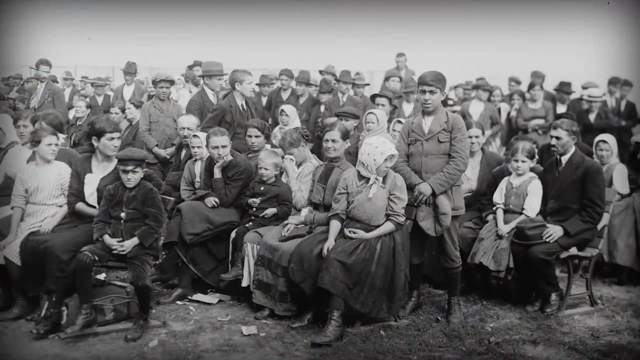 Of course, by the end of the 19th century, immigration was not a new phenomenon in the United States. After the first wave of colonization by English people and Spanish people and other Europeans, there was a new wave of Scandinavians, French people and especially the Irish. 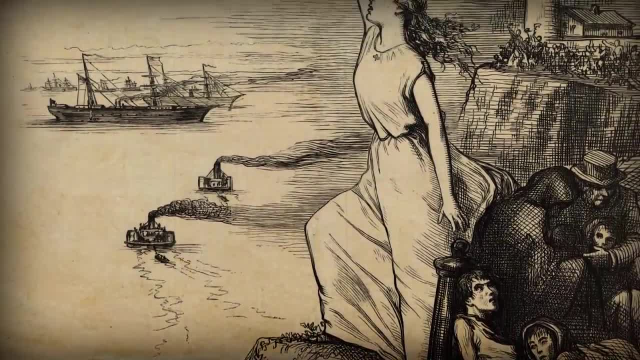 Most of you probably know about the potato famine of the 1840s that led a million Irish men and women to flee into the US. So the first wave of colonization of the United States was the first wave of colonization of the United States. 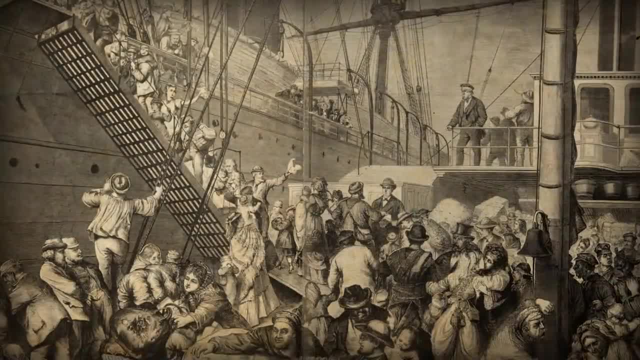 So the first wave of colonization was the first wave of colonization of the United States. If you don't know about it, it was awful. And the second largest wave of immigrants was made up of German speakers, including a number of liberals who left after the abortive revolutions of 1848. Alright, let's go to the Thought Bubble. The Irish had primarily been farmers in the motherland, but in America they tended to stay in cities like New York and Boston. Most of the men began their working lives as low-wage, unskilled laborers, but over time they came to have much more varied job opportunities. 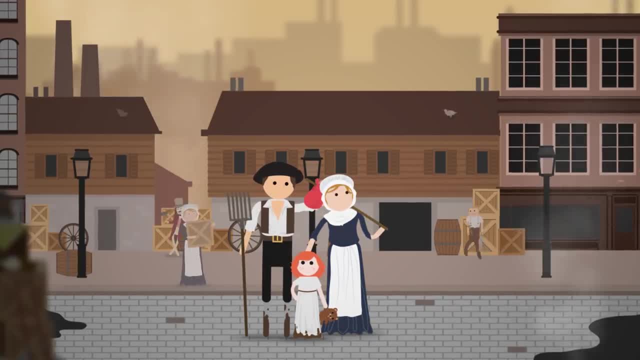 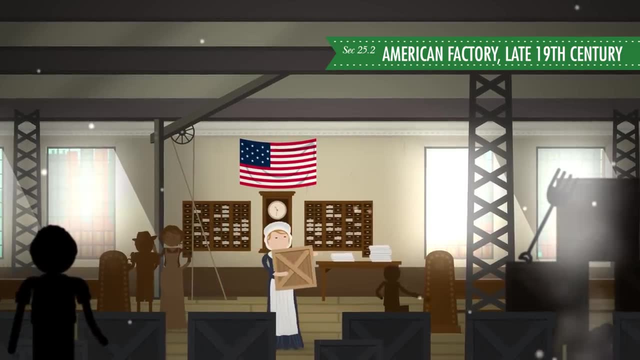 Irish immigrant women worked too, some in factories or as domestic servants in the homes of the growing upper class. Many women actually preferred the freedom that factory labor provided, and one Irish factory woman compared her life to that of a servant by saying: Our day is ten hours long, but when it's done, it's done and we can do what we like with. 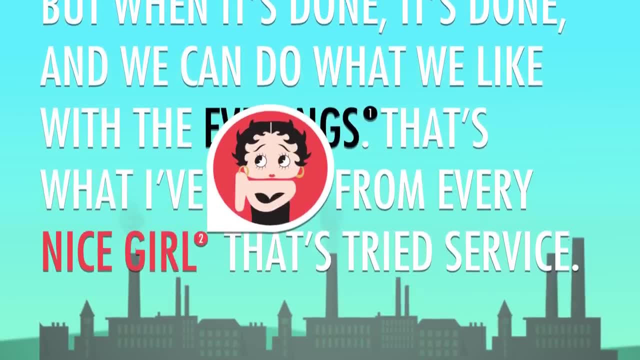 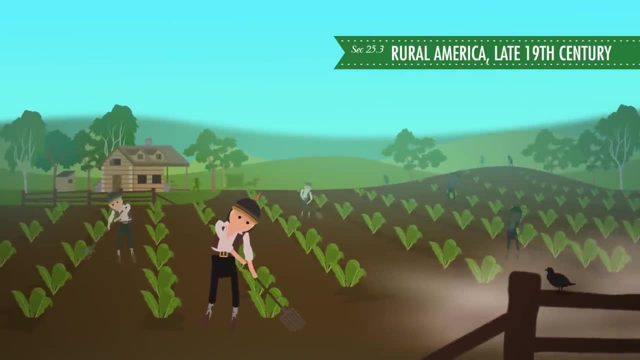 the evenings. That's what I've heard from every nice girl that's tried service. You're never sure that your soul is your own, except when you're out of the house. Most German speakers had been farmers in their home countries and would remain farmers in. 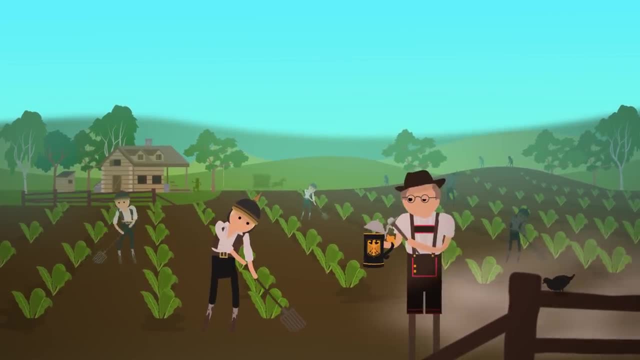 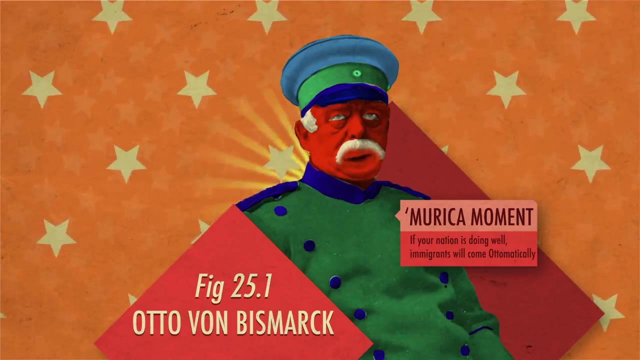 the US, but a number of skilled artisans also came. They tended to stay in cities and make a go of entrepreneurship. Bismarck himself saw emigration from Germany as a good thing, saying The better it goes for us, the higher the volume of emigration, And that's why we named 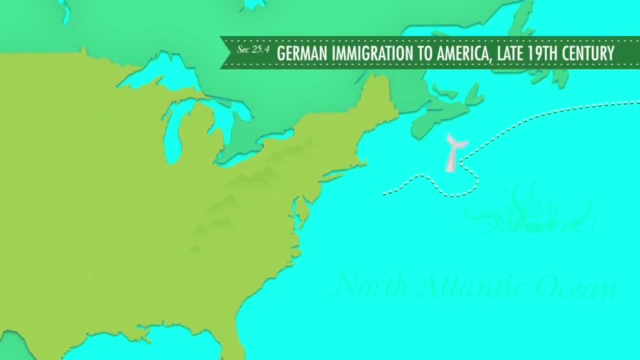 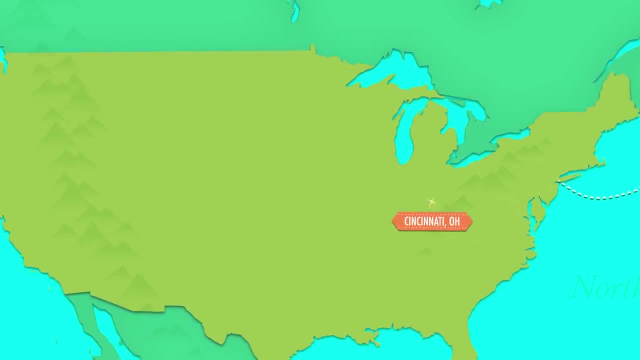 a city in North Dakota after him. Although enough German immigrants came to New York that the Lower East Side of Manhattan came to be known for a time as Kleindeutschland- Little Germany, many moved to the growing cities of the Midwest, like Cincinnati and St Louis, Some of the most famous German 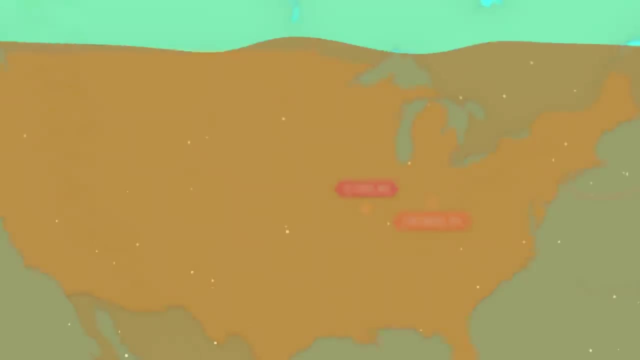 immigrants became brewers. and America is much richer for the arrival of men like Frederick Pabst, Joseph Schlitz and Adolphus Busch- And by richer I mean German immigrants, And by richer I mean German immigrants- And America is much richer for the arrival of men like Frederick Pabst, Joseph Schlitz and Adolphus Busch. 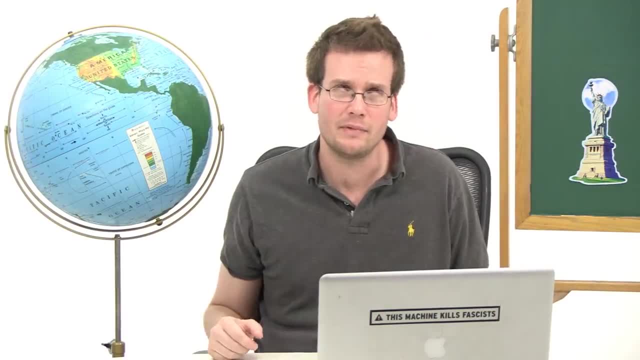 And by richer I mean German immigrants, And America is much richer for the arrival of men like Frederick Pabst, Joseph Schlitz and Adolphus Busch. Hey, thanks for not ending on a downer Thought Bubble. I mean, unless you count alcoholism. 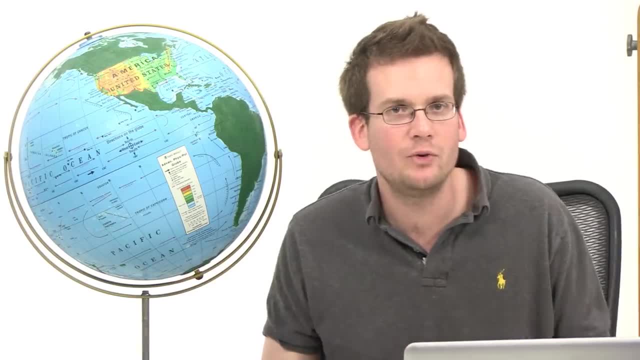 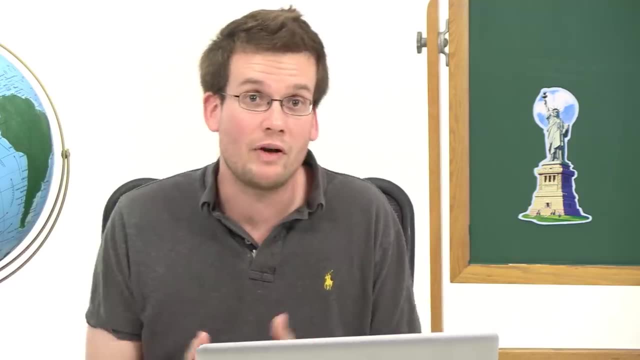 So, but by the 1890s over half of the 3.5 million immigrants who came to our shores came from southern and eastern Europe, in particular Italy and the Russian and Austro-Hungarian empires. They were more likely than previous immigrants to be Jewish or Catholic, and while almost all of them were looking for work. many were also escaping political or religious persecution, And by the 1890s they also had to face new scientific theories, which I'm putting in air quotes to be clear, Because there was nothing scientific about them which consigned them to different races. 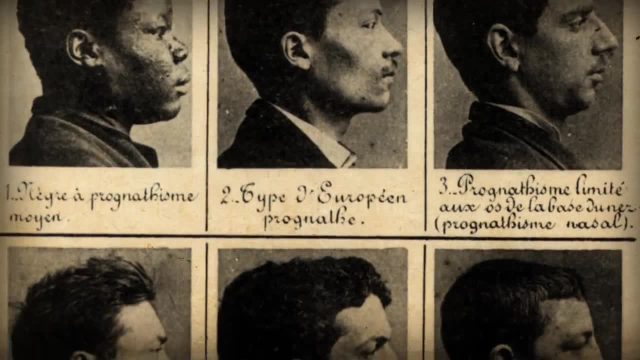 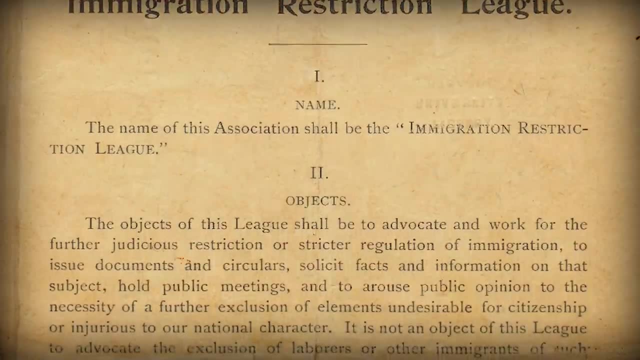 whose low level of civilization was fit only for certain kinds of work and predisposed them to criminality. The Immigration Restriction League was founded in Boston in 1894 and lobbied for national legislation that would limit the number of immigrants, and one such law even passed Congress. 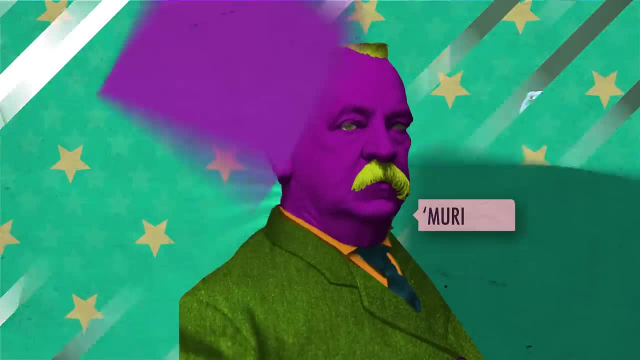 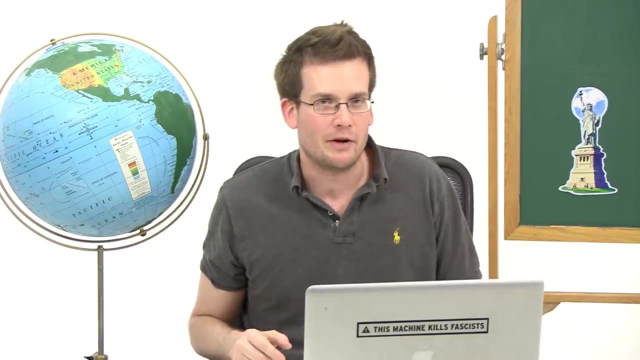 in 1897, only to be vetoed by President Grover Cleveland. Good work, Grover. You know his first name was Stephen, but he called himself Grover. I would have made a different choice, But before you get too excited about Grover Cleveland, Congress and the President were. 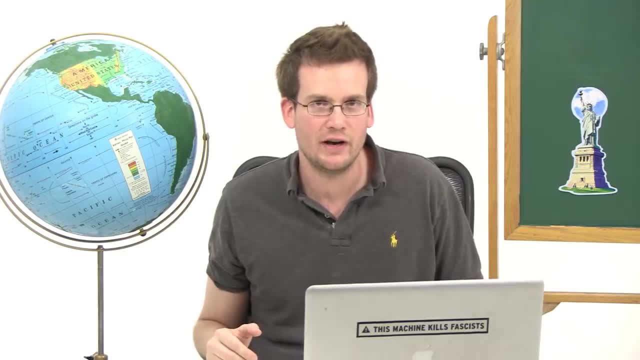 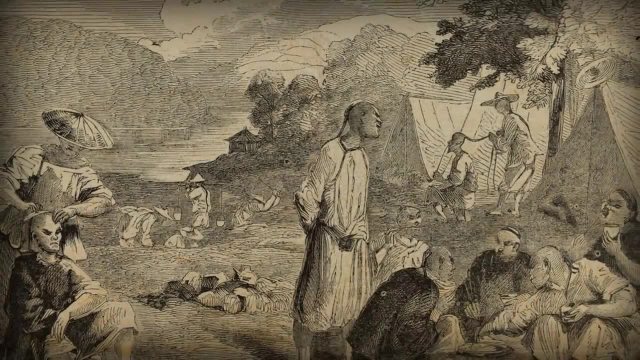 able to agree on one group of immigrants to discriminate against the Chinese. Chinese immigrants, overwhelmingly male, had been coming to the United States, mostly to the West, since the 1850s to work in mines and on the railroads. They were viewed with. suspicion because they looked different, spoke a different language and they had strange habits like regular bathing. By the time the Chinese Exclusion Act went into effect in 1882, there were 105,000 people of Chinese descent living in the United States, mainly in cities on the West Coast and in 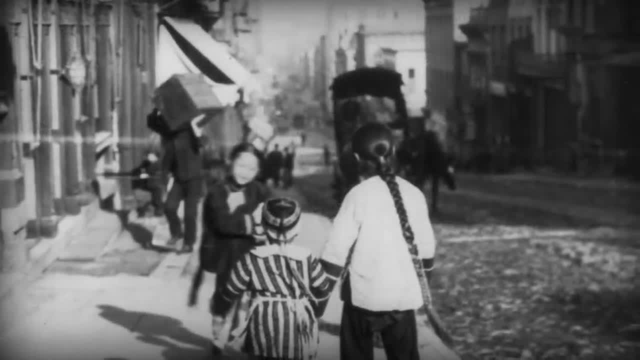 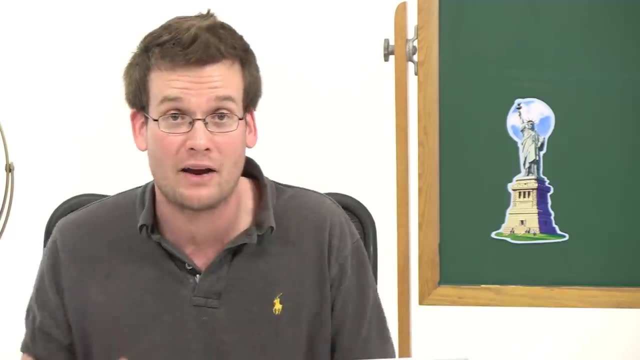 the West Coast. San Francisco refused to educate Asians until the state Supreme Court ordered them to do so, And even then the city responded by setting up segregated schools. The immigrants fought back through the courts. In 1886, in the case of Yick Woe v Hopkins, the United States Supreme Court ordered San 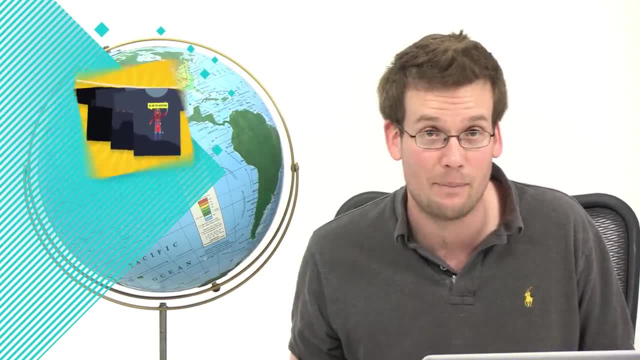 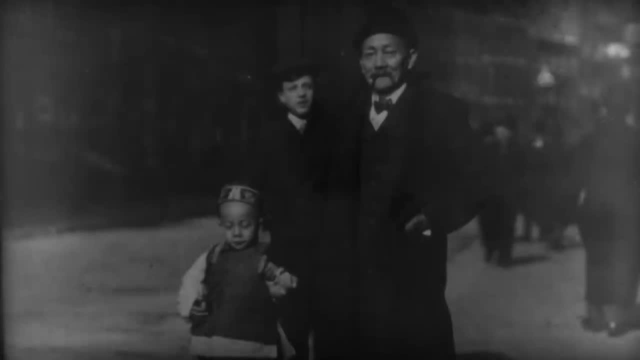 Francisco to grant Chinese-operated laundries licenses to operate. Then, in 1898, in United States v Wong Kim Ark, the court ruled that American-born children of Chinese immigrants were entitled to citizenship under the 14th Amendment, which should have: 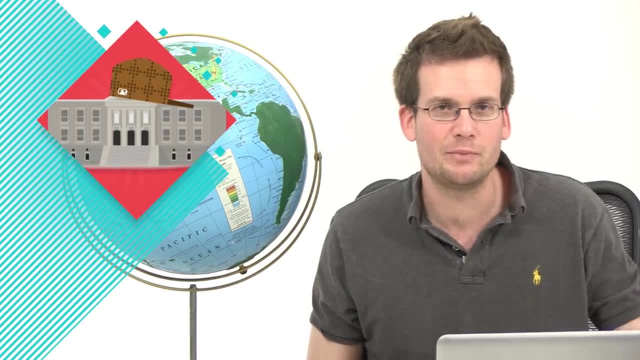 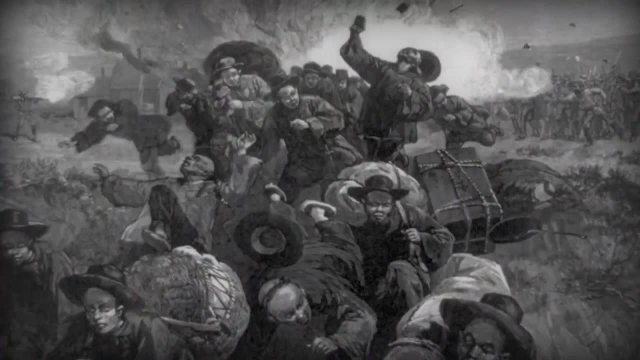 been a duh, but wasn't. We've been hard on the Supreme Court here at Crash Course, but those were two good decisions. You go, Supreme Court. But despite these victories, Asian immigrants continued to face discrimination in the form of vigilante-led riots, like the one in Rock Springs, Wyoming, that killed 26 people and 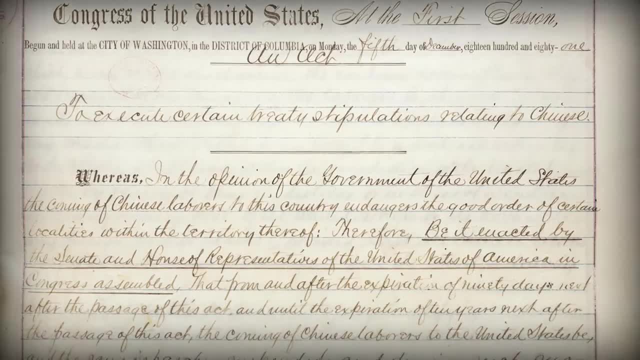 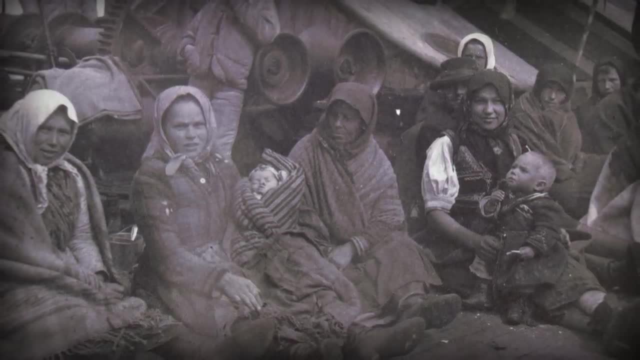 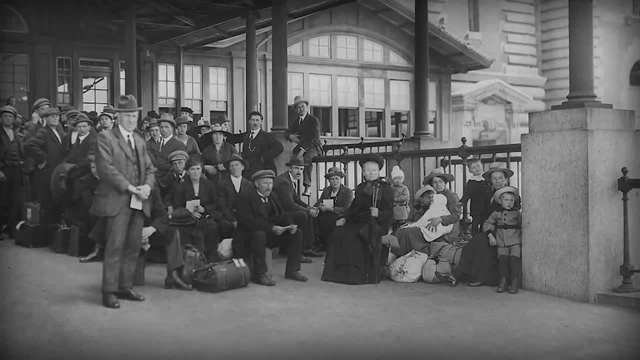 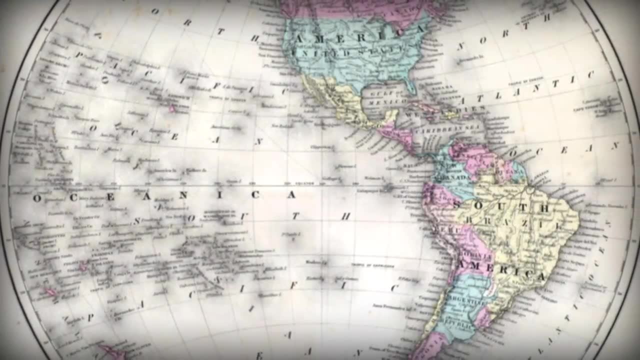 1914, 13 million immigrants came to the United States. In the entire period touched off by the industrialization, from 1840 until 1914, a total of 40 million people came to the US, But at least 20 million people emigrated to other parts of the Western Hemisphere, including. Brazil, the Caribbean, Canada- yes, Canada- and Argentina. As much as we have Italian immigrants to thank for things like pizza- and we do thank you- Argentina can be just as grateful for the immigrant ancestors of Leo Messi, Also the. 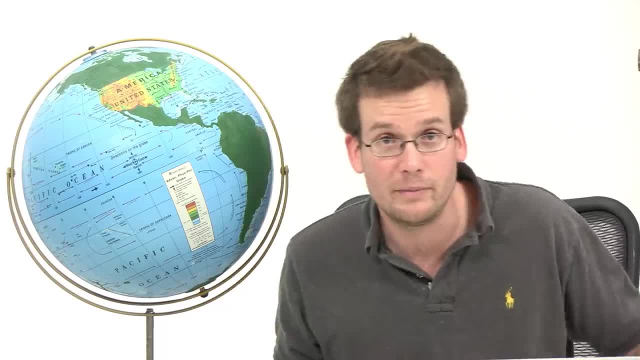 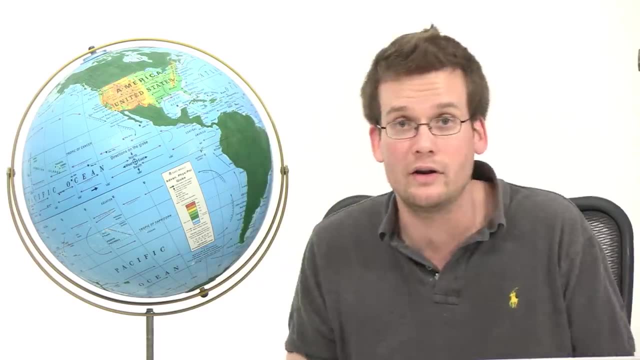 Pope, although he has never once won La Liga. There was also extensive immigration from India to other parts of the British Empire like South Africa, Chinese immigration to South America and the Caribbean. I mean, the list goes on and on. In short, America is not as special as it fancies itself. 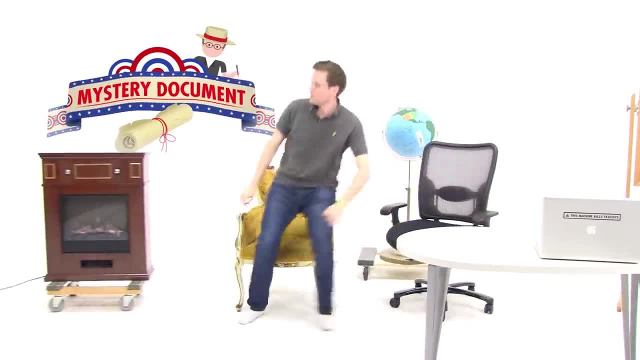 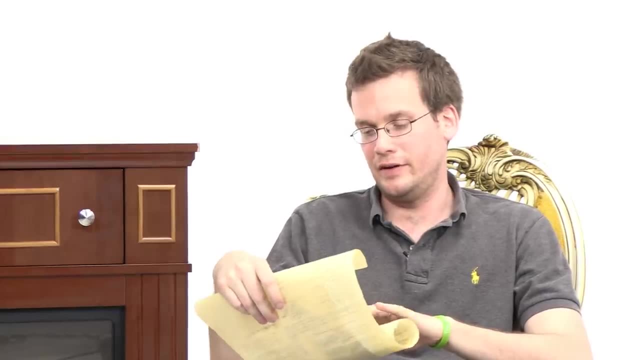 Oh, it's time for the mystery document. The rules here are simple. I guess the author of the mystery document. I get it wrong and then I get shocked with the shock pen. Sorry, I don't mean to sound defeatist, but I don't have a good feeling about this. 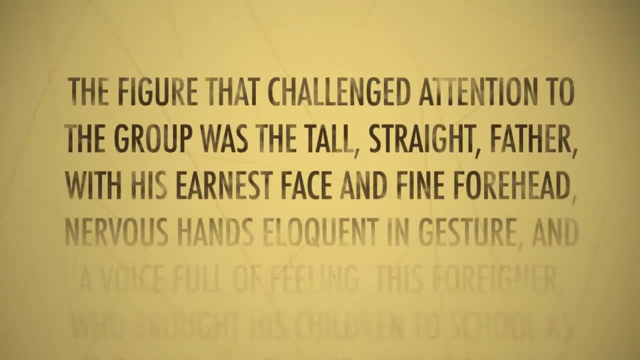 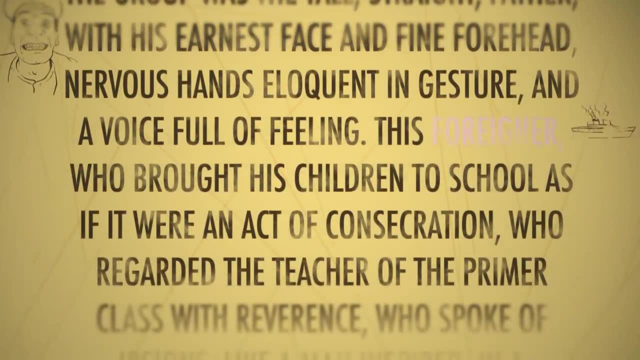 All right. The figure that challenged attention to the group was the tall, straight father with his earnest face and fine forehead. nervous hands eloquent in gesture and a voice full of feeling. This foreigner who brought his children to school as if it were an act of consecration. 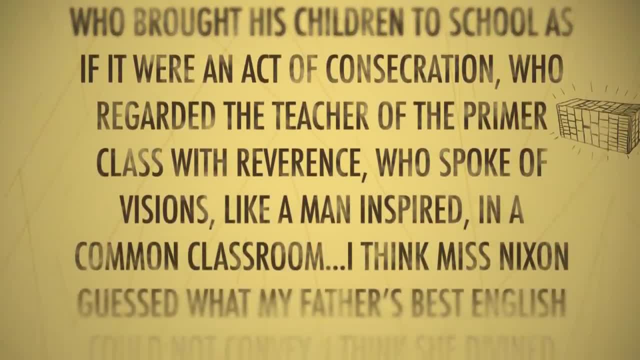 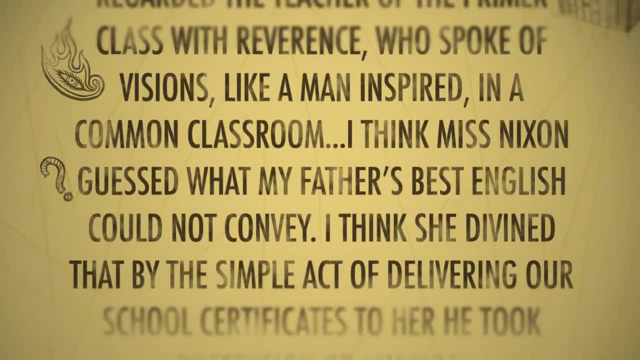 who regarded the teacher of the primer class with reverence, who spoke of visions like a man inspired in a common classroom. I think Ms Nixon guessed what my father's best English could not convey. I think she divined that by the simple act of delivering our school certificates to her. 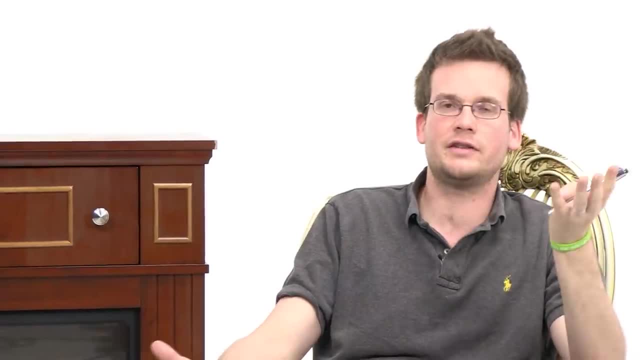 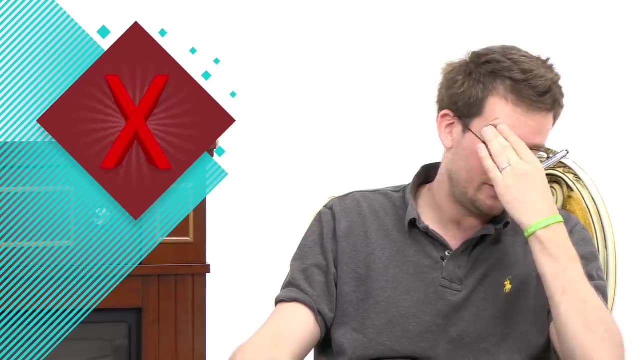 he took possession of America. Uh, I don't know. At first I thought it might be someone who works with immigrants like Jane Addams, but then at the end, suddenly it's her own father. Jane Addams' father was not an immigrant. 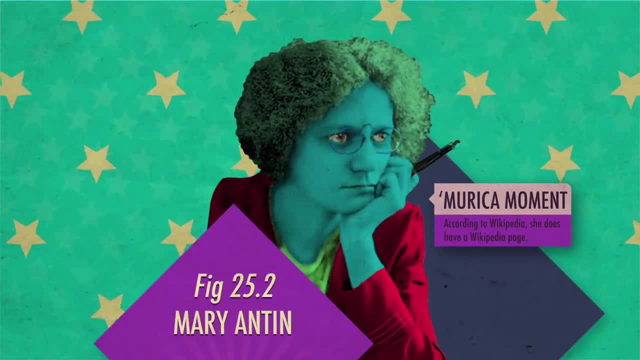 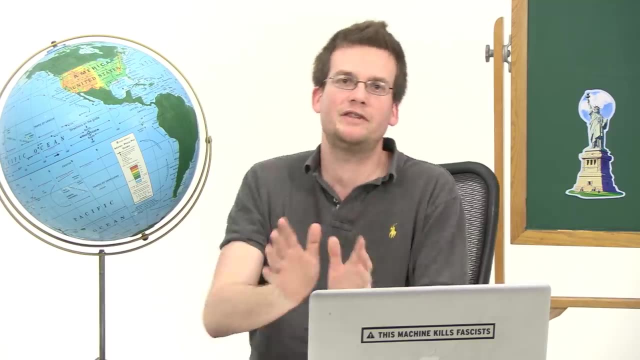 Mary Anton, Does she even have a Wikipedia page? She does. Did you write it, Stan? Stan wrote her Wikipedia page. So this document, while it was written by someone who should not have a Wikipedia page, points out that most immigrants to America were coming for the most obvious reason: opportunity. 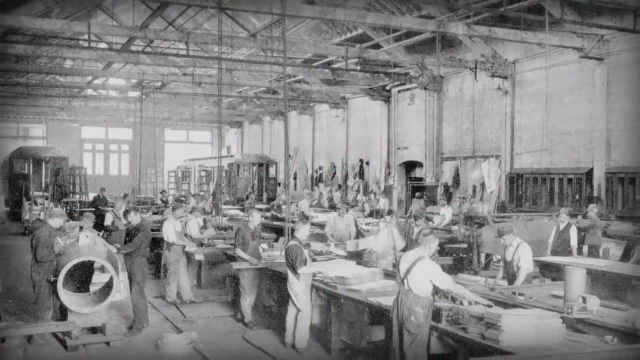 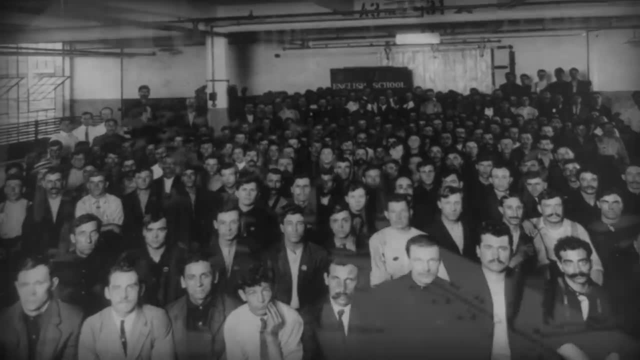 Industrialization, both in manufacturing and agriculture, meant that there were jobs in America. There was so much work, in fact, that companies used labor Labor recruiters who went to Europe to advertise opportunities. Plus, the passage was relatively cheap, provided you were only going to make it once in your 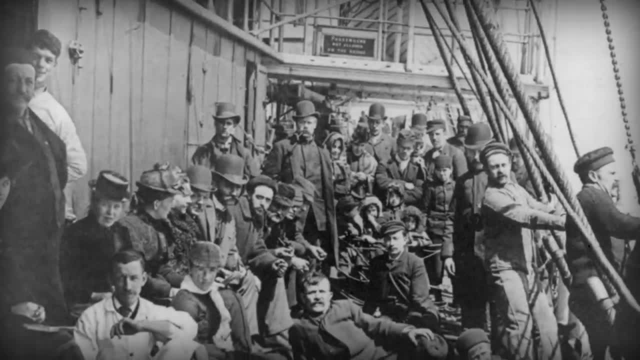 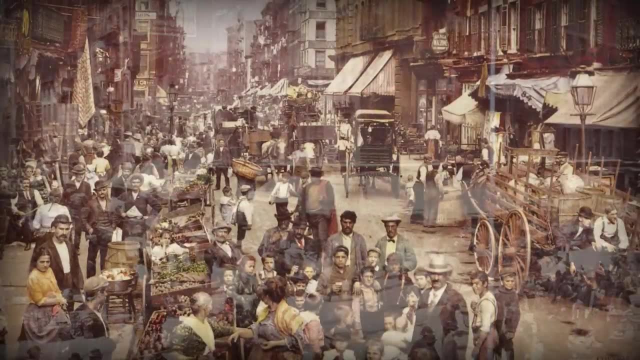 life, and it was fast, taking only eight to twelve days on the new steam-powered ships. The Lower East Side of Manhattan became the magnet for waves of immigrants, first Germans, then Eastern European Jews and Italians, who tended to recreate towns and neighborhoods within blocks and sometimes single buildings. 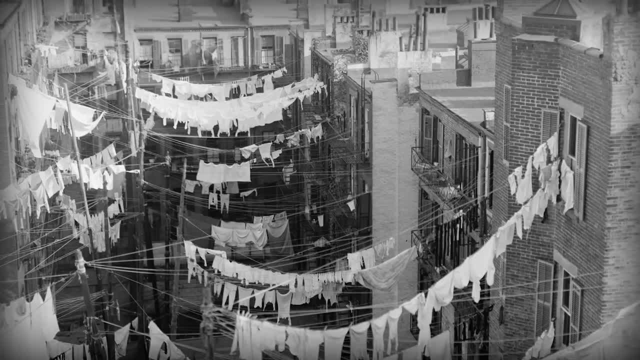 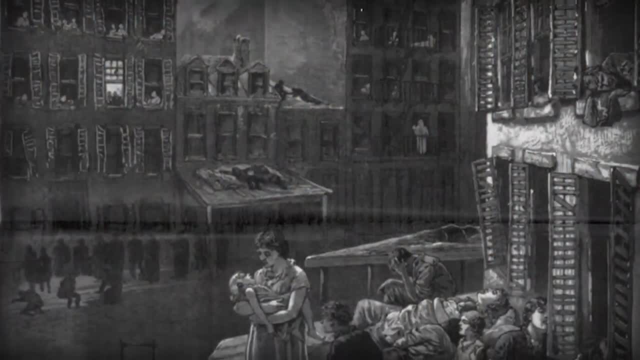 Tenements. these four- five- and six-story buildings that were designed to be apartments sprang up in the second half of the nineteenth century, and the earliest ones were so unsanitary and crowded that the city passed laws requiring a minimum of light and ventilation. And often these tenement apartments doubled as workspaces because many immigrant women and children took in piecework, especially in the garment industry. Despite local laws mandating the occasional window and outlawing the presence of cows on public streets, conditions in these cities were pretty bad. 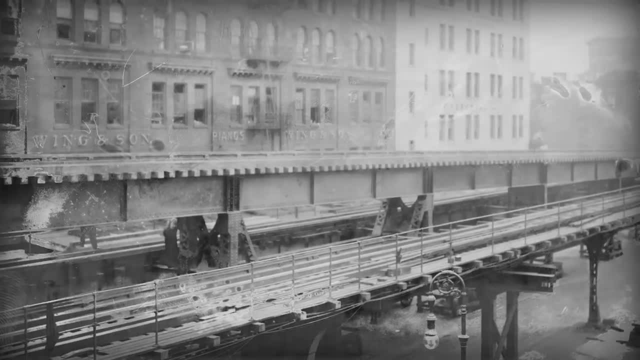 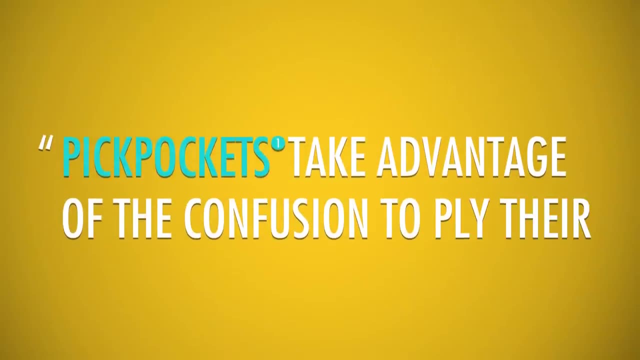 Things got a little bit better with the construction of elevated railroads and later subways. that helped relieve traffic congestion, but they created a new problem: Pickpockets. Pickpockets take advantage of the confusion to ply their volutes. Pickpockets. 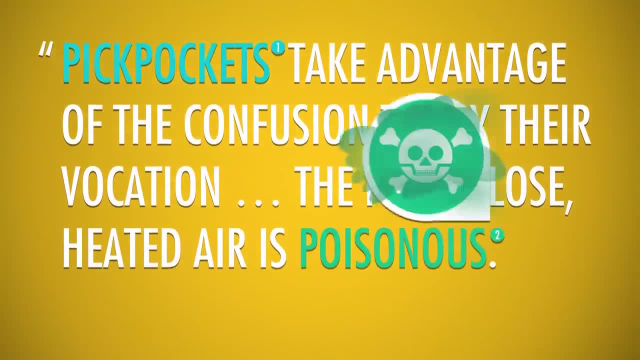 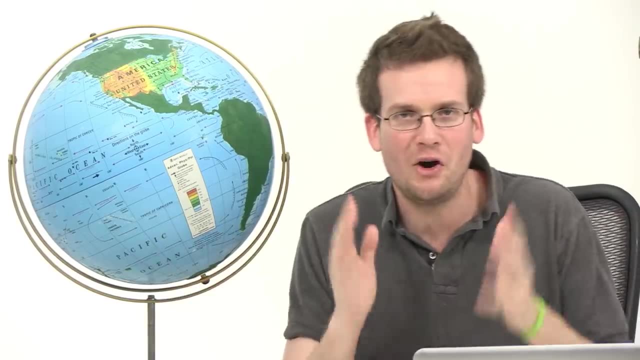 Pickpockets are always in the right location, The foul close. heated air is poisonous. A healthy person cannot ride a dozen blocks without a headache, So that's changed. This new transportation technology also enabled a greater degree of residential segregation in cities. 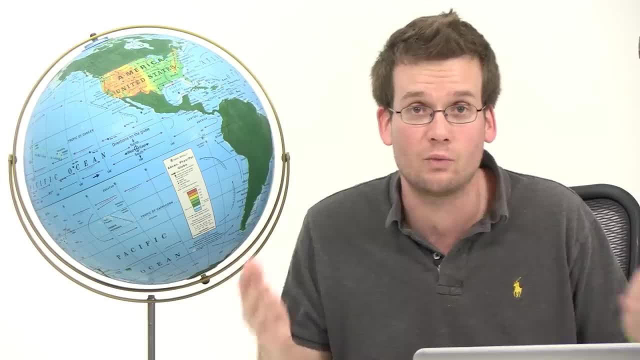 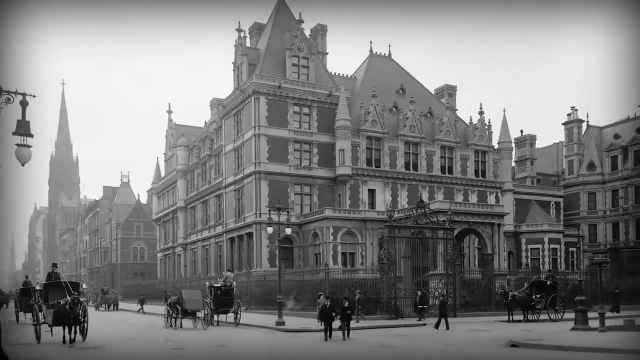 Manhattan's downtown area had at one time housed the very rich as well as the very poor, But improved transportation meant that people no longer had to live and work in the same place. The wealthiest, like Cornelius Vanderbilt and JP Morgan, constructed lavish palaces. 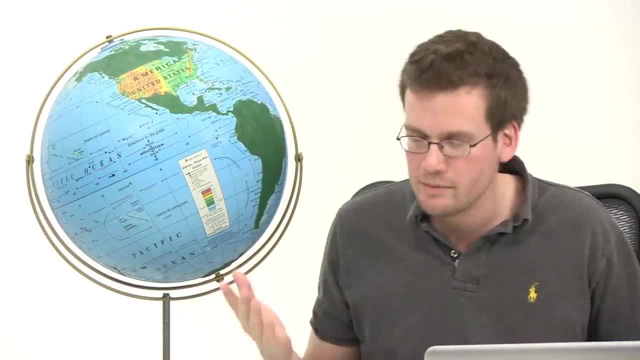 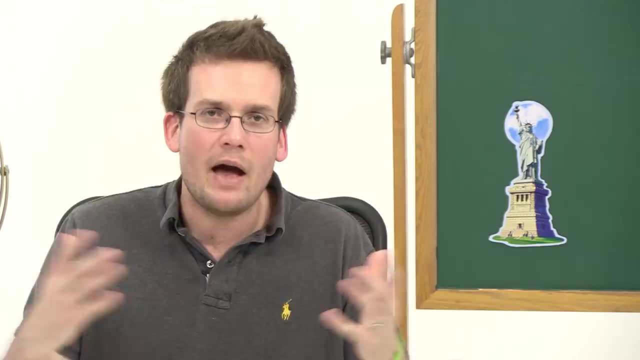 for themselves. Uptown townhouses were common, But until then, one of the most notable features of Gilded Age cities like New York was that the rich and the poor lived in such close proximity to each other, And this meant that with America's growing urbanization, the growing distance between 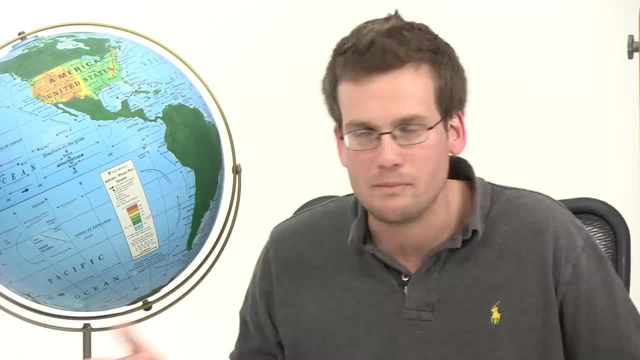 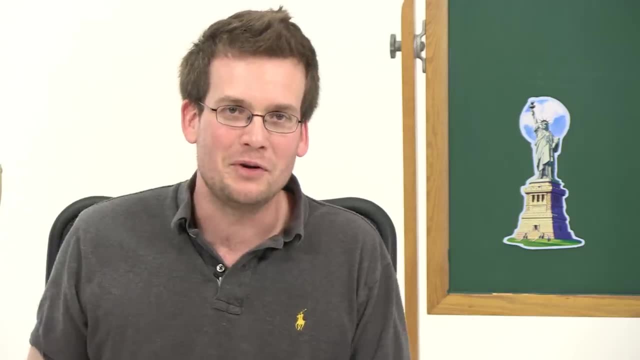 rich and poor was visible to both rich and poor, And much as we see in today's megacity. this inability to look away from poverty and economic inequality became a source of concern. Now, one way to alleviate such concern is to create suburbs, so you don't have to look. 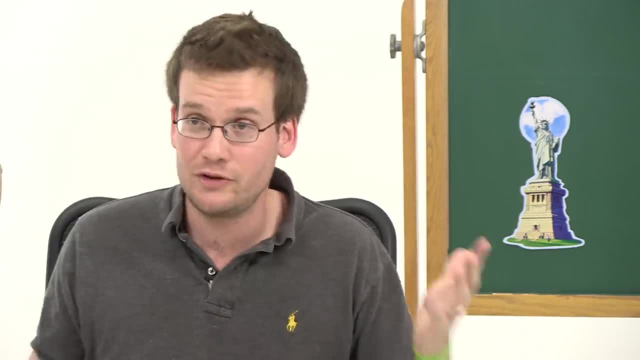 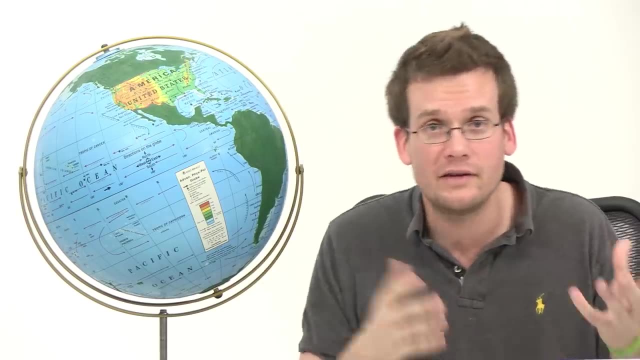 at poor people. But another response to urban problems was politics, which in cities like New York became something of a contact sport. Another response was the so-called Progressive Movement. And in all these responses and in the issues that prompted them, urbanization, mechanization. 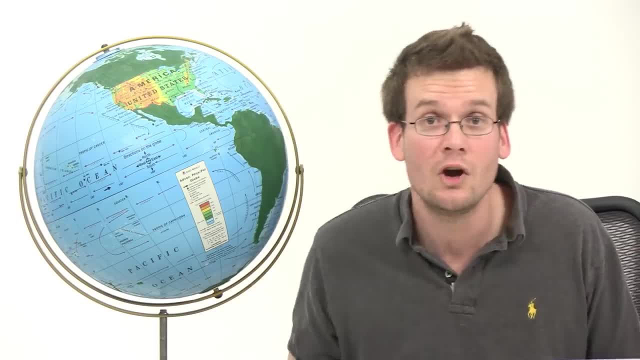 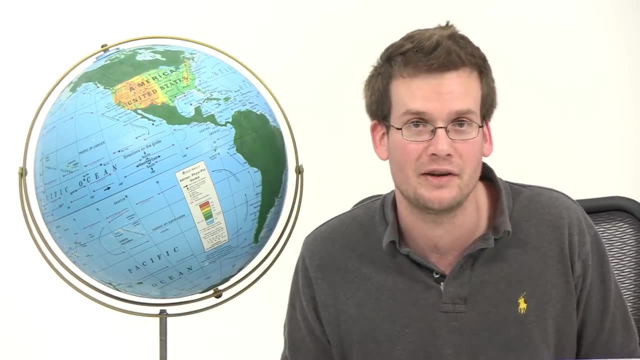 capitalism, the distribution of resources throughout the social order. we can see modern, industrial America taking shape, And that is the America we live in today. Thank you for watching. I'll see you next week. Crash Course is produced and directed by Stan Muller. 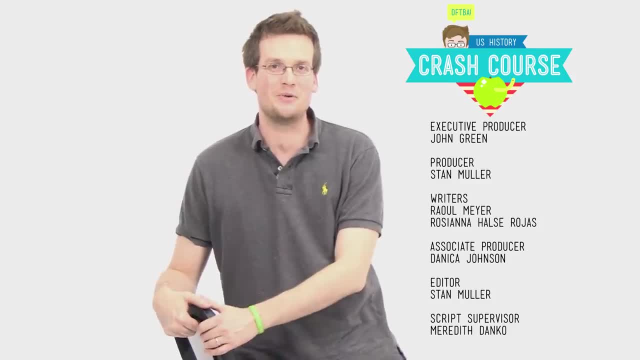 The script supervisor is Meredith Danko. The show is written by my co-host, Dan Mullen. This is my high school history teacher, Raul Meyer, Rosianna Rojas and myself. Our associate producer is Danica Johnson, and our graphics team is Thought Cafe. 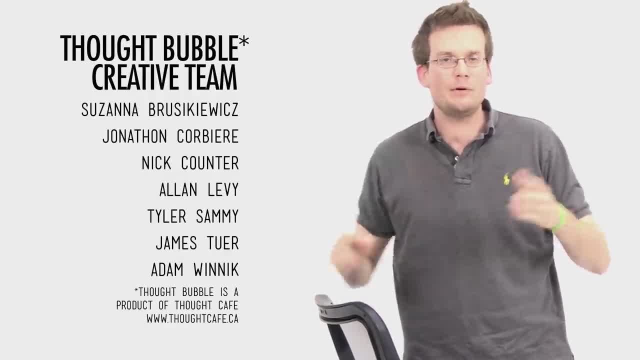 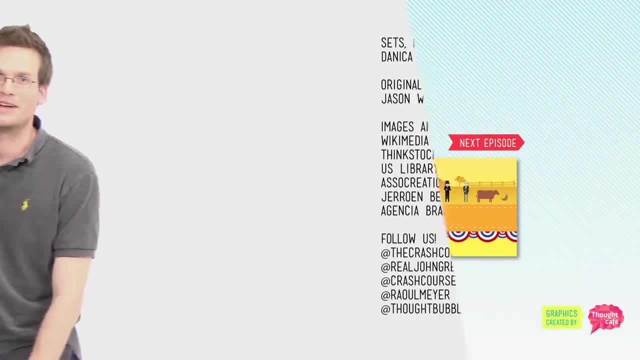 Every week, there's a new caption for the Libertage. If you'd like to suggest one, you can do so in comments, where you can also ask questions about today's video. that will be answered by our team of historians. Thank you for watching Crash Course and, as we say in my hometown, don't forget to be. awesome.